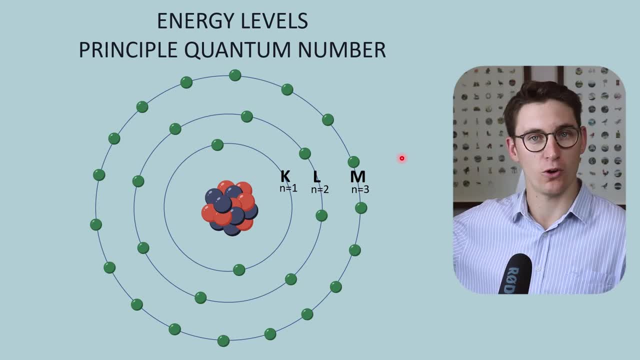 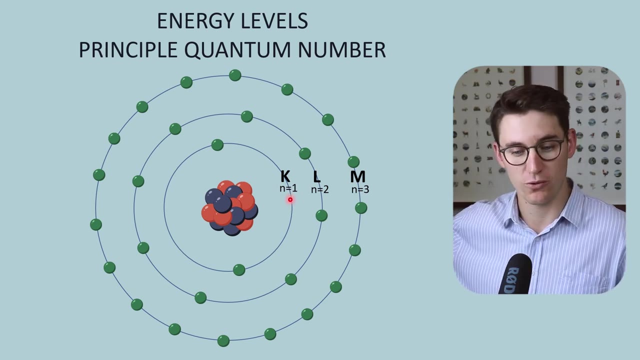 letter K, and we work our way out L, M, N, O, P. We can also label these with these: N equals to one, N is the quantum number or the principal quantum number of that energy level. And we start with one and again work our way out: N equals two, three, four and so on, And this is what's. 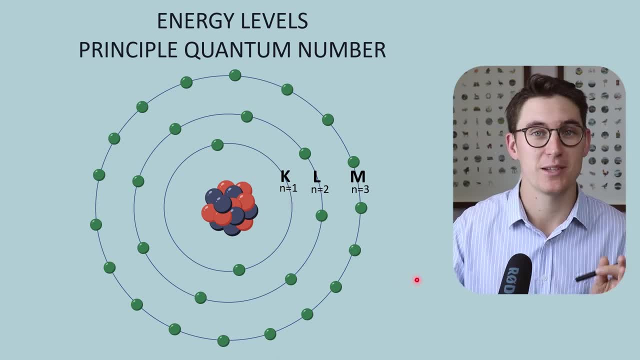 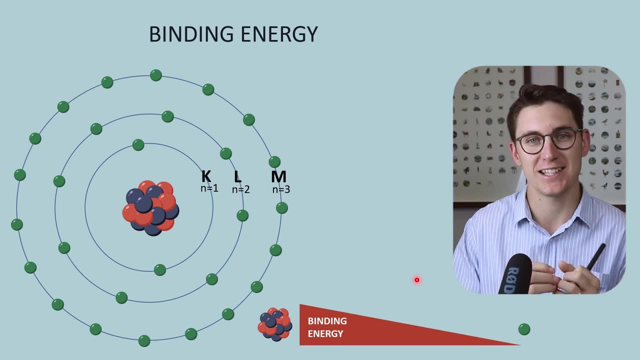 known as the principal quantum number. Now, perhaps the most important concept when it comes to energy levels is this concept of binding energy. Binding energy is the energy required to release an electron from the atom itself. Now, binding energy is dependent on two things. One, the electron's proximity to the nucleus. The closer that electron is to the 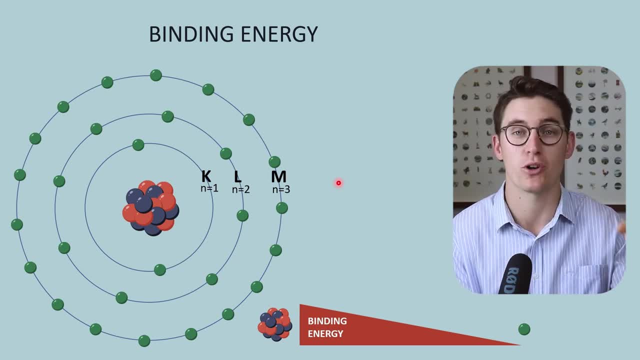 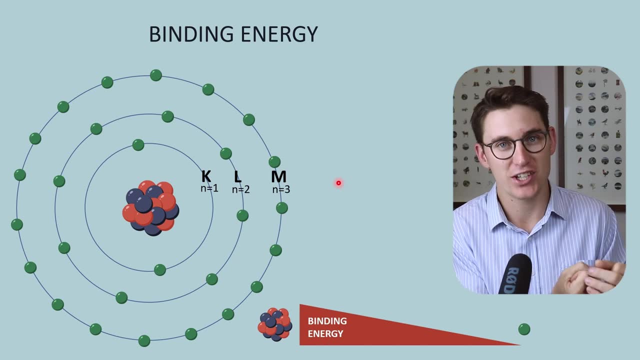 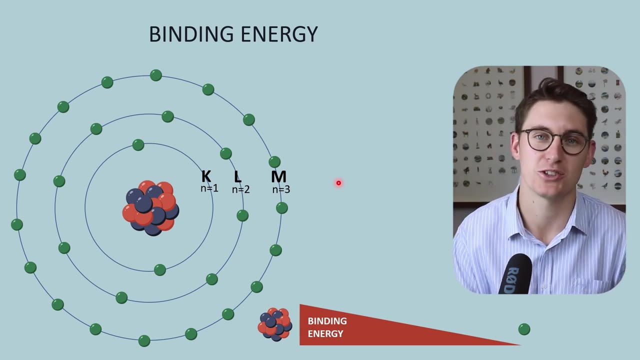 atom's nucleus, the stronger that force of attraction between the positive protons and that negative electron, That stronger force of attraction, the binding energy, the energy that is required to release that electron from the atom, gets stronger as that electron gets closer in proximity to the nucleus. The second dependent factor is the number of protons within the nucleus. 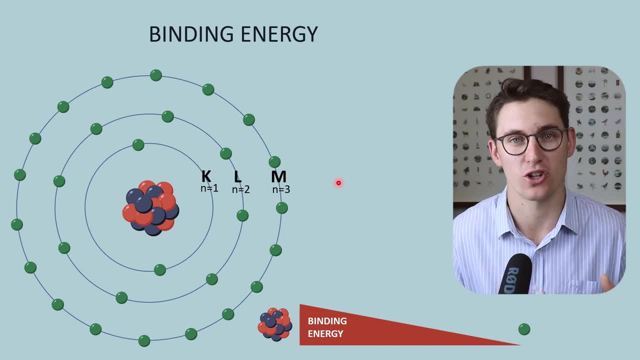 of that electron. The second dependent factor is the number of protons within the nucleus of that atom. The more protons, the more positive charge, the stronger that force of attraction to the electrons in the various different energy levels. So binding energy gets stronger as we get closer. 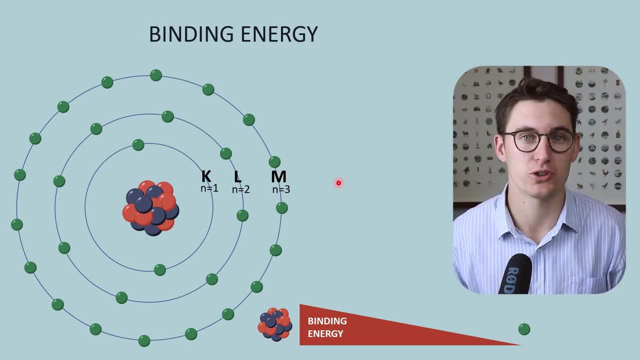 to the nucleus and it gets stronger. as we increase our number of protons within the nucleus- And you'll see, when we look at x-ray physics, this binding energy becomes particularly important because in order to create certain types of x-rays, we need to eject an electron from an atom. 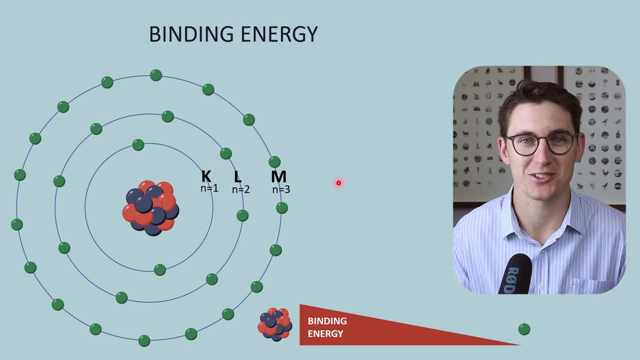 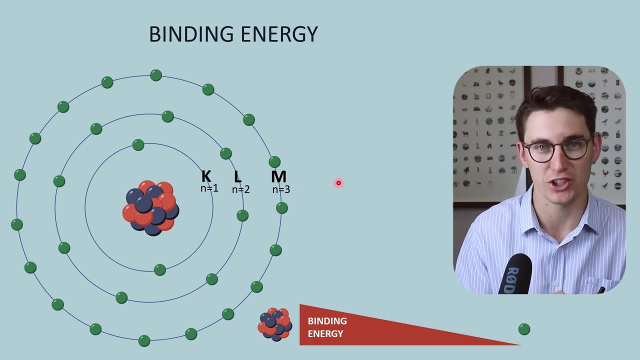 first, in order to create what is known as a characteristic x-ray, which we're going to look at in our x-ray physics module. So this concept of binding energy is incredibly important. Our K-shell binding energies are always going to be more than our L-shell and the L-shell energies. 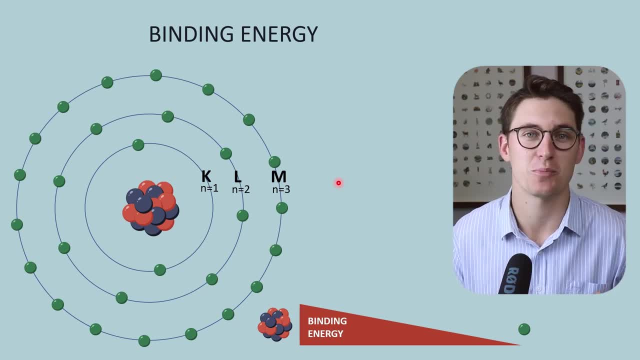 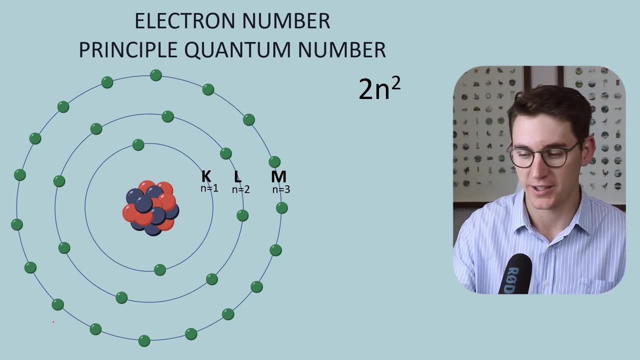 will be more than our M-shell respectively, And it's the difference in those binding energies that helps us to create what is known as characteristic x-ray. So if we go back now to our principal quantum number, the number that we've labeled each one of these energy levels, we can use that. number in order to Vergleich each energy level of the shell, and we can do this step-by-step. that would be known as the characteristic x-ray Lets. beginning with the looks of nature, the one we know is going to be used as our biggest energy, And I'll be expressing it in 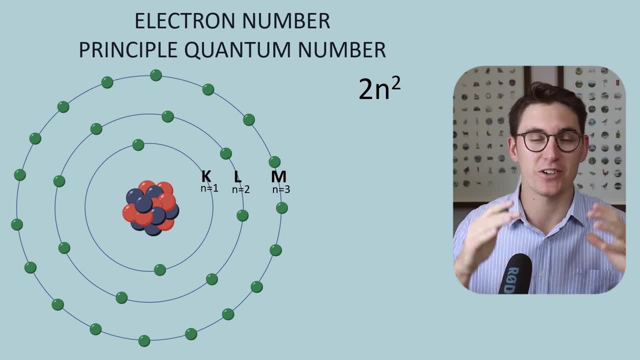 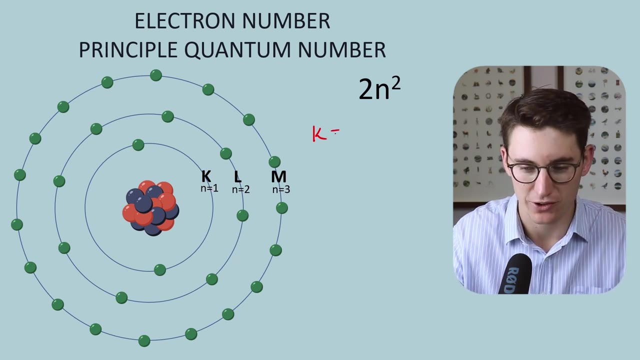 to then determine the number of electrons that that specific shell can house. and the way we do that is by using this formula here: 2n to the power of 2. so if we look at our k shell here, our k shell has a quantum number of 1, so the number of electrons that our k shell can house is 2 times. 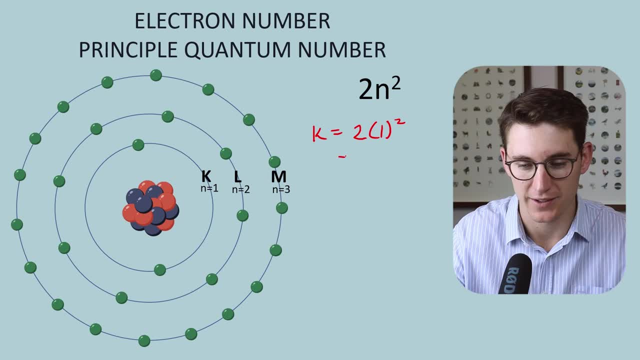 1 to the power of 2. 1 to the power of 2 is 1. the number of electrons in our k shell will be 2. you can see there are 2 electrons here in our l shell. our principal quantum number is 2, so our 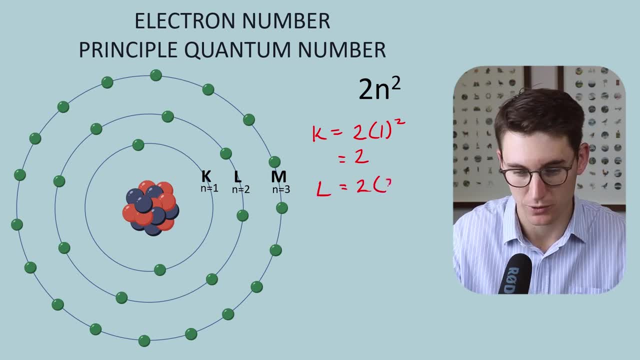 l shell can house 2 times our principal quantum number, which is 2 to the power of 2. this is 4. 2 times 4 is 8. there are 8 electrons within our l shell. our m shell, then, can house more electrons. so let's have a look at our m shell. our principal quantum number here is 3. 3 to the power of 2 is 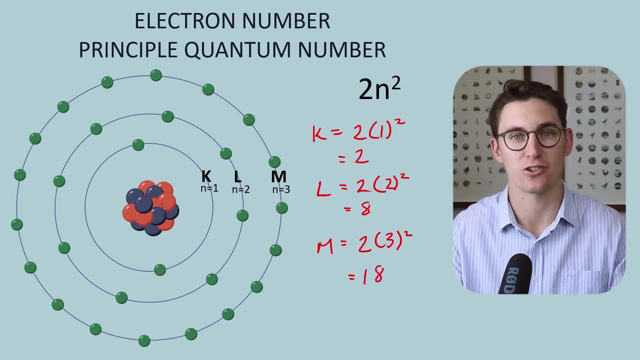 9 times 2 equals 18. we can get 18, 2, 4, 18 electrons within our m-shell. So you can see the larger atoms that have more energy levels can house more and more electrons in those further out LMNO electron shells And what is responsible. 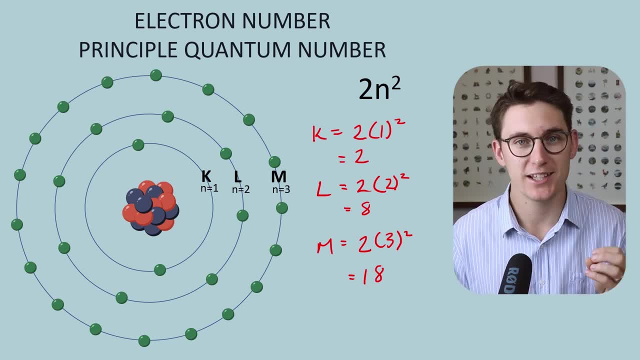 for these numbers. the number of electrons within each shell is our electron orbitals. Now, just while we're here and before you move on, if you are here, I assume you're either starting your radiology physics journey or you're coming back to revise your radiology physics, And I've 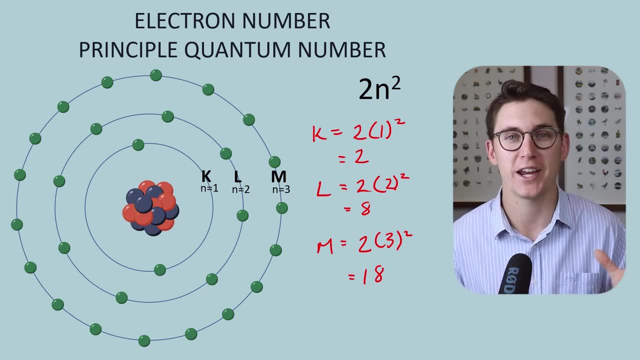 created a resource in the first line of the description where I've curated a bunch of past paper questions and I've gone ahead and answered those past paper questions in depth through videos like this. And so if you're interested in that, if you got a radiology physics exam coming up, 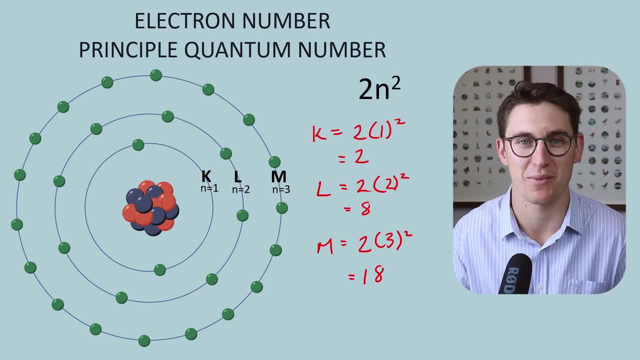 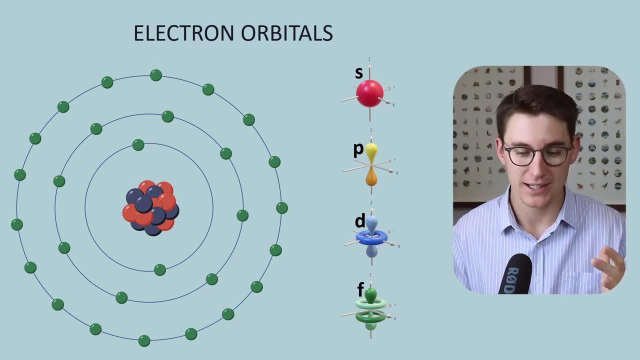 I'd really appreciate it if you go and check out that course. I've put a lot of time and effort into it. Now there are four different types of electron orbitals. We have an s-orbital, a, p, a, d and an f-orbital. Now, what exactly is an? 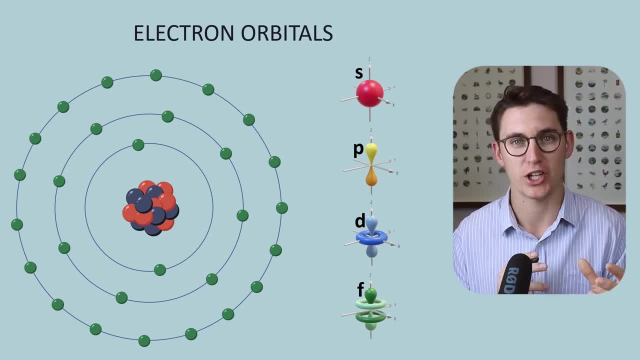 electron orbital. Well, an electron orbital, as you can see here, is a 3D shape and it's a region of probability or likelihood of an electron occurring in that 3D space within an atom. So electrons don't necessarily go in perfect circles around the nucleus, They actually exist. 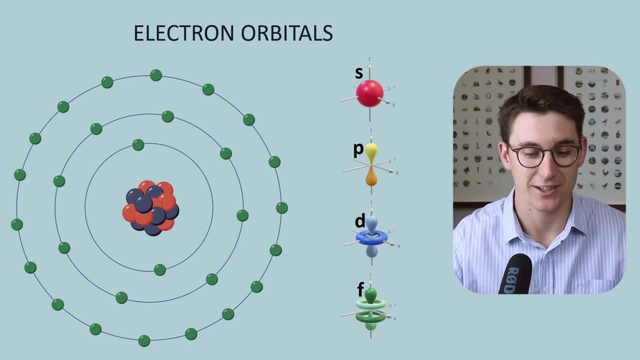 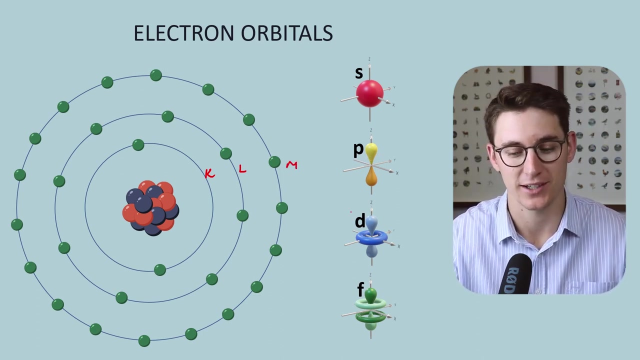 within these various different shapes. Now, as we start at our K shell, here we have only one type of orbital and that is our S orbital. Moving on to the L shell, we have both an S orbital and a P orbital. Our M shell has an S, a, P and a D, and as we extend further out, we add these orbitals in. 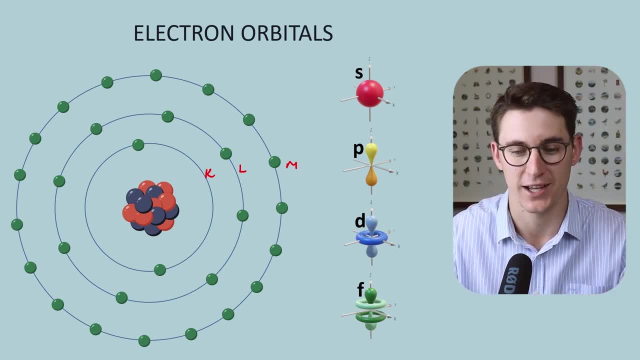 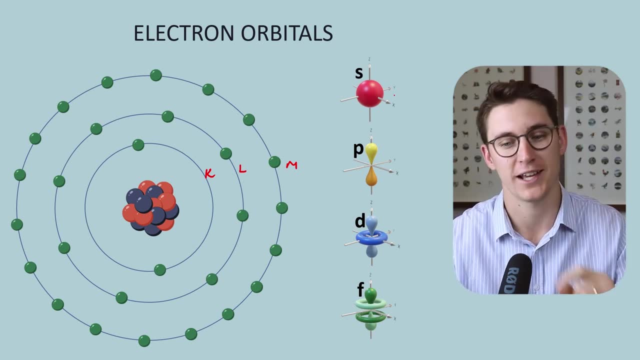 Now, each of these orbitals can house a specific number of electrons, and electrons will always come in pairs within these orbitals. So our S orbital can hold one electron pair, so two electrons in total. Our P orbital can hold three electron pairs, or six electrons in total. Our D orbital can hold 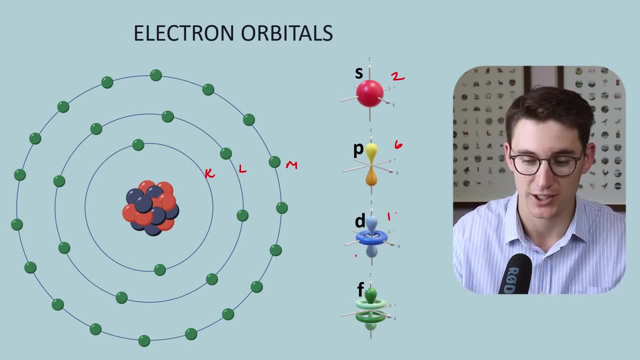 five electron pairs, that is, 10 electrons in total, and our F is seven electron pairs, or 14 electrons in total. So let's have a look. We said our K shell has two electrons within its orbital. Our K shell only has an S orbital and that's where our 2 comes from. Our L shell has 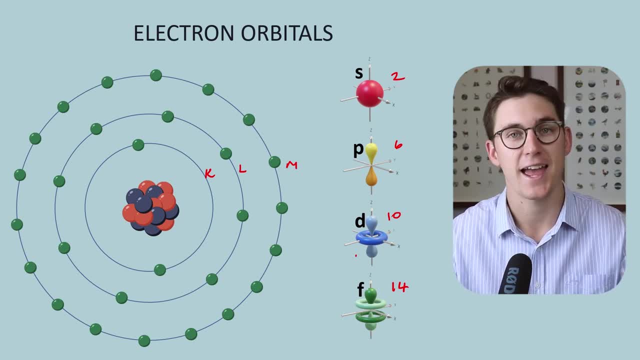 both an S orbital and an S orbital, and that's where our 2 comes from. Our L shell has both an S and a P orbital. It's got two plus six, eight electrons. Our M shell also has D orbitals, so we've 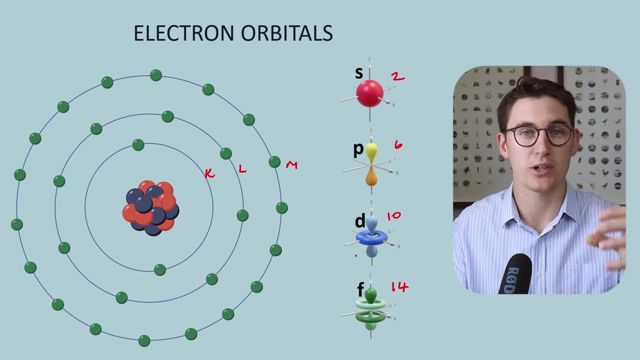 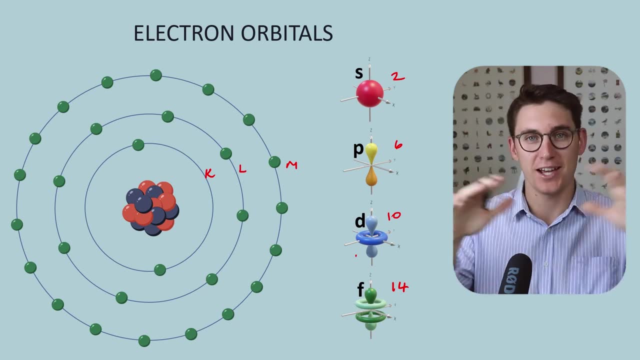 got two, six, ten, eighteen electrons, and that's what we calculated with our principal quantum number. So you can see that our classic understanding of how electrons go in these electron shells is slightly more complex when we start to look at electron orbitals Now. 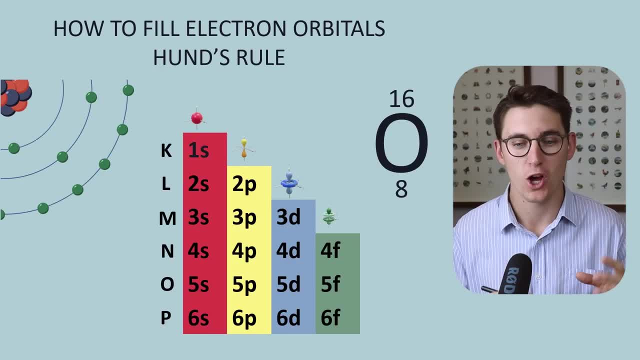 we can go about determining how to fill those electron orbitals when we're looking at a specific atom. So let me take a moment here to describe this graph to you here. Each one of these rows here determines a different electron shell, our K shell, L, M, N, as we extend out. 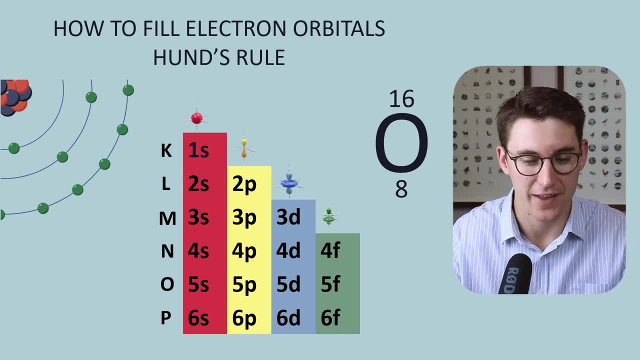 The columns represent the types of electron orbitals and the numbers here are our principal quantum numbers. So we can see our K shell has only got an S orbital. L has got S P, M has got S P D, just as we've looked at in the previous slide. 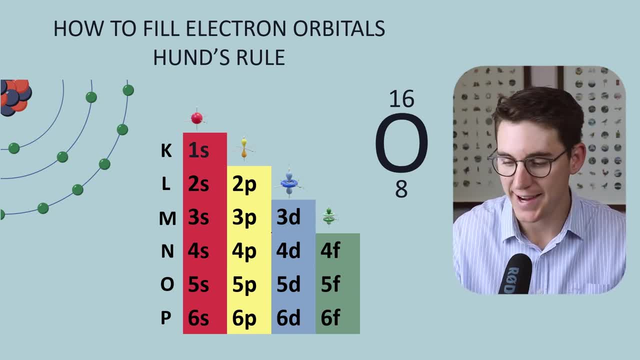 Now, if we were to take oxygen, for example, our oxygen has eight protons. here We've seen this before. Our atomic number is eight, eight protons, Our mass number is 16, so we've got eight protons and eight neutrons. and assuming that this oxygen was uncharged, we would have: 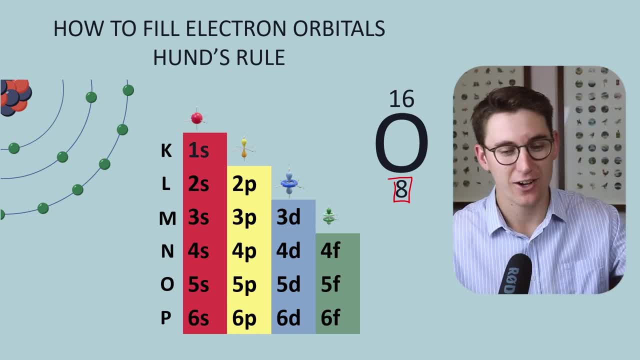 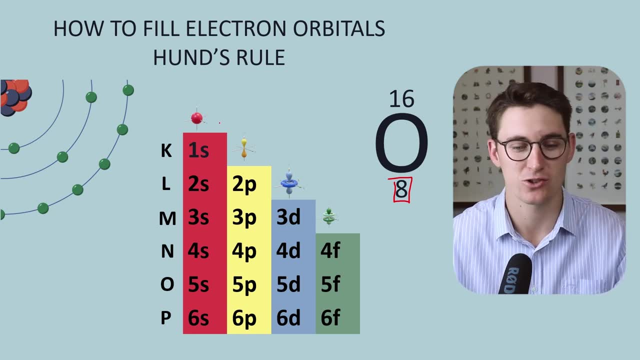 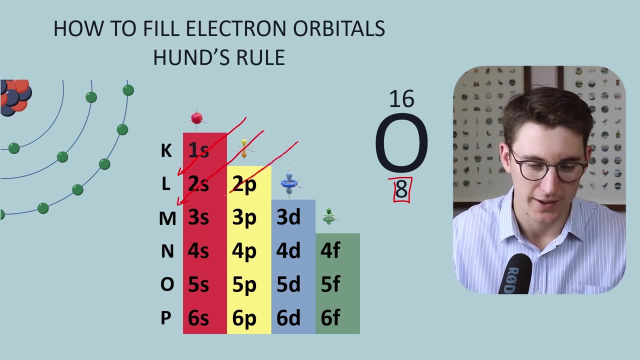 eight electrons. So our eight electrons now need to fit into our electron orbitals, And the way we go about filling these electron orbitals is what is known as Hund's rule. We draw a diagonal through these orbitals like this, And these diagonal lines determine the order in which we 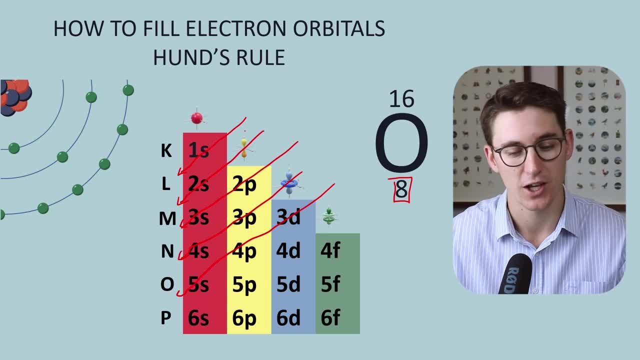 fill these orbitals. So you can see as we go down, like this: we start at one S orbital, then our two S, two P and three S, three P and four S, and so on as we go down. So let's go about pitting these. 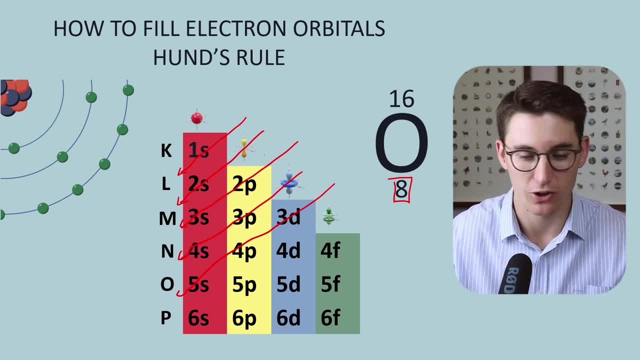 eight electrons into these electron orbitals. We know that our S orbital can house two electrons: our P six and our P eight. So we know that our S orbital can house two electrons: our P six, our D 10, and our F 14.. So we've got eight electrons to play with. So our first two go into. 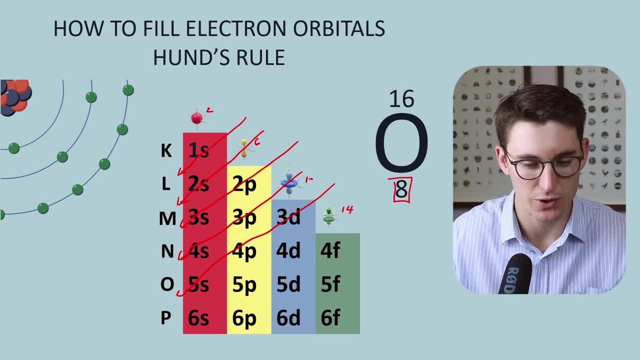 this one S orbital. Our second two then go into our two S orbital. We've now got four electrons left and our P orbital can house a total of six electrons. So the four electrons can fill into this P orbital. So this is the outermost orbital within our atom and this is what's known as our valence. 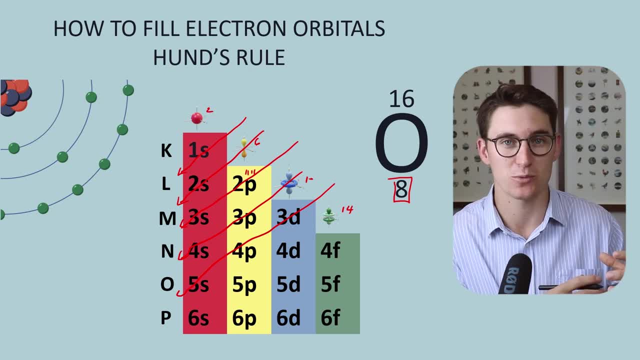 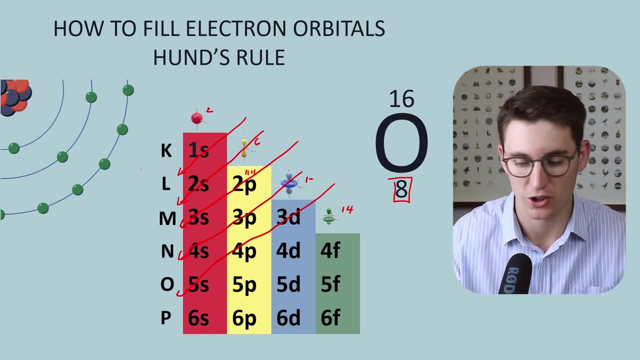 electrons, a really important concept when it comes to determining how atoms will react to other atoms, how atoms will react to external forces. So here, when we're describing oxygen, we can describe it as a two P four, a two P four. Our quantum number of two in the P orbital has four valence.